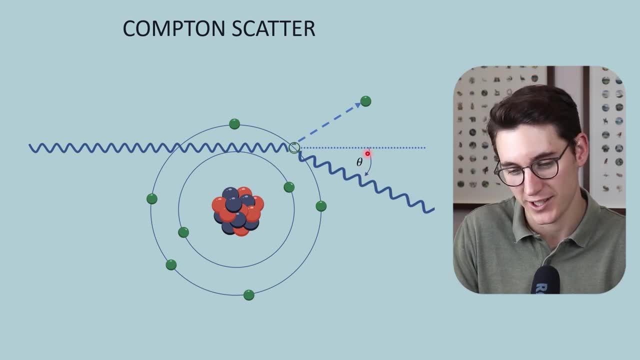 incident x-ray and our scattered x-ray here. This theta here represents our scatter angle. Now this photoelectron will have an energy that is proportional to the scatter angle. The larger the scatter angle here of this Compton scattered x-ray, the larger the energy, or the more the energy of this photoelectron. 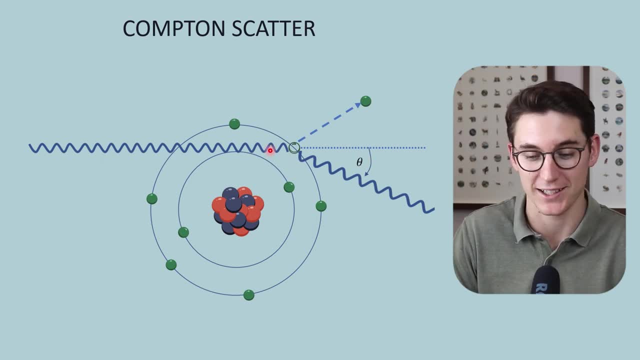 This energy of this Compton scatter is determined by the incident energy and the scatter angle here. Now you may be wondering: what about the binding energy here? Well, in tissues, our valence electrons, the binding energy is so small that it's actually inconsequential in these calculations. 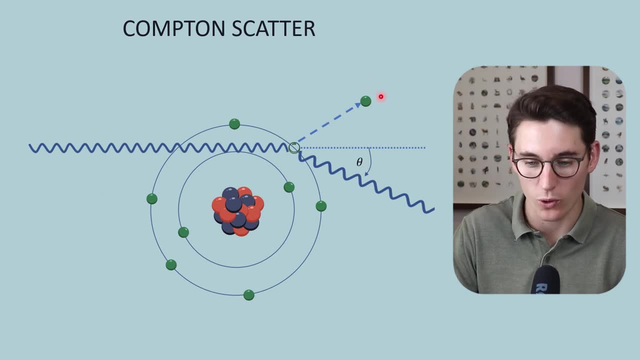 What we need to know is the larger the scatter angle, the more energy that's been conferred to this photoelectron and the less energy this Compton scatter has. So as we increase the scatter angle, we decrease the energy of this Compton scatter. You can think about it as a billiard ball. If we 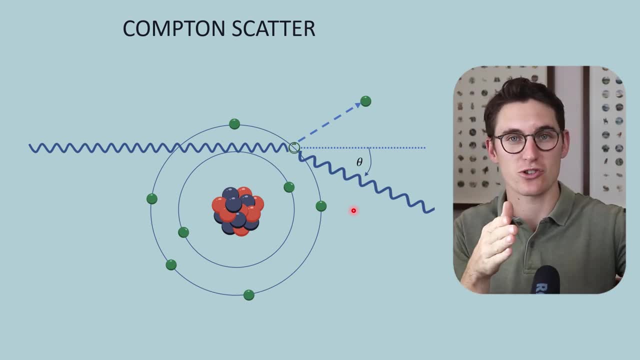 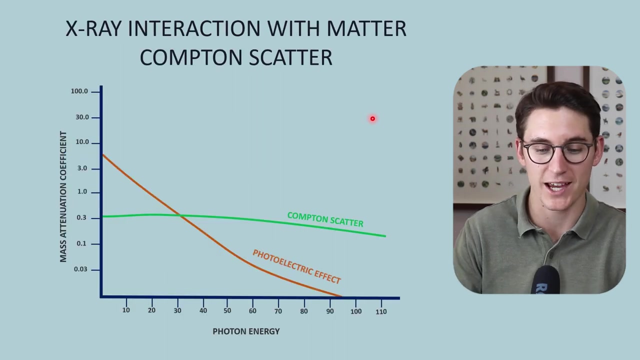 have a glancing blow. very little of that energy has been transferred to the photoelectron. If we have a large collision with a high scatter angle, we lose a lot of energy in that collision and most of that energy is released in the form of this photoelectron's kinetic energy. Now again we can. 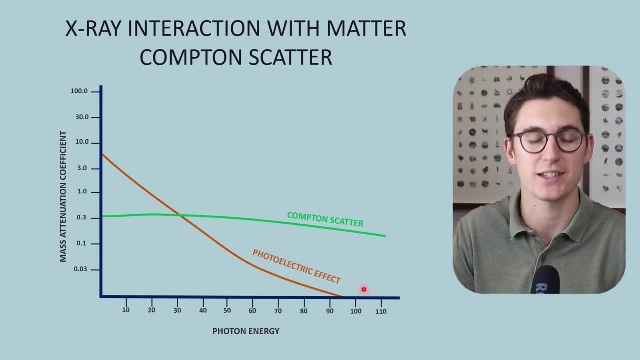 draw this on a graph and you'll see that Compton scatter is quite different to the photoelectric effect. In the photoelectric effect we saw the likelihood of the photoelectric effect decreasing exponentially with increasing photon energy. We know that in a more dense tissue this 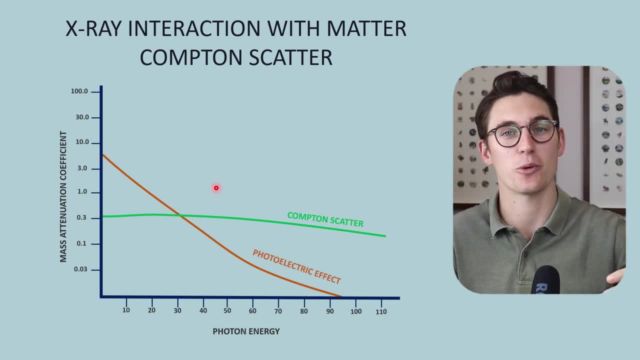 photoelectric effect will increase and in a higher atomic number tissue the photoelectric effect will increase even further. Now Compton scatter in diagnostic energy ranges has very little dependence on incident x-ray energy, unlike photoelectric effect. There's a very small decrease in the amount of Compton scatter. that happens as we increase our incident photon energy. 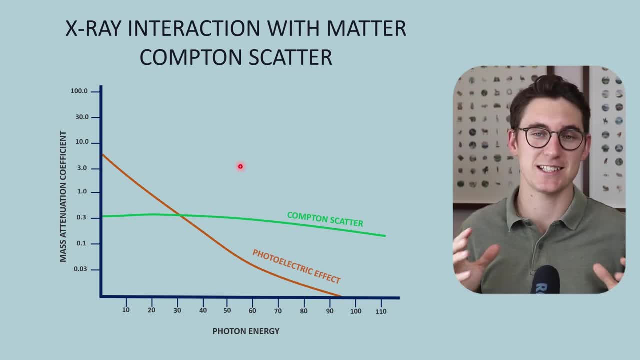 Compton scatter's likelihood is largely dependent on the density of the tissue or the electron density within that tissue. It has very little to do with atomic number, because as our atomic number increases so does our number of electrons and that electron density remains roughly equal. So Compton scatter is largely dependent on density, has very little.